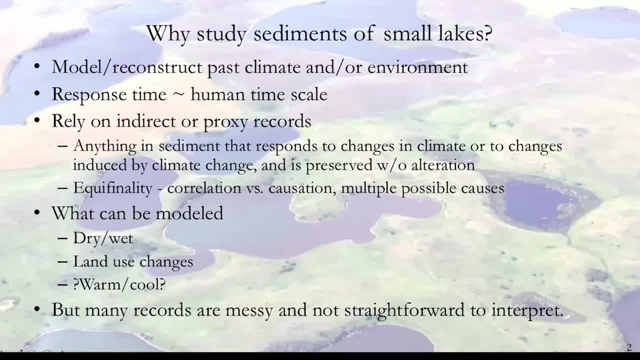 use changes And in some other locations it is possible to model what its warm or cool. okay, The many records are quite messy and it's not straightforward to interpret And it's a big contrast to some of the well known paleo-climate records such as deep sea record, such as the. benthic stack. I'm sharing the second radar. This is from the intercontinental ocean record, the best perspective and it's very good. But if you look at the high-altitude records, we have some of the best examples in the ocean report and we have some of the most important records, but we do take 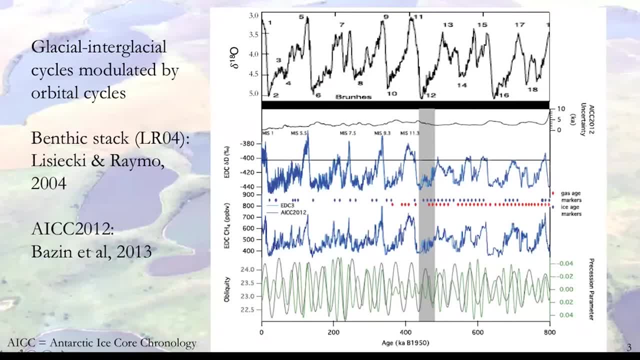 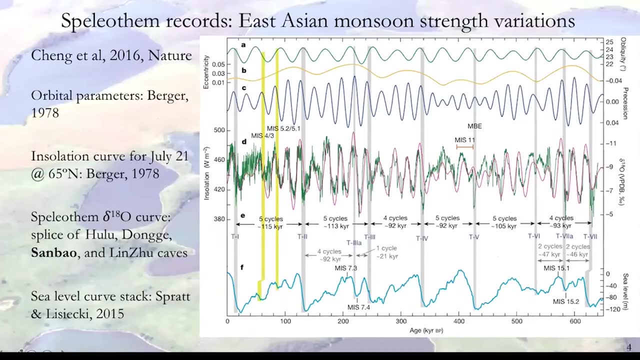 in Raymo 2004,. or Antarctic ice core record, which shows the glacier integration cycles, or some of the Spirothem records. I'm showing one from Hai Cheng 2016 paper and his co-authors. So East Asia monsoon regions. 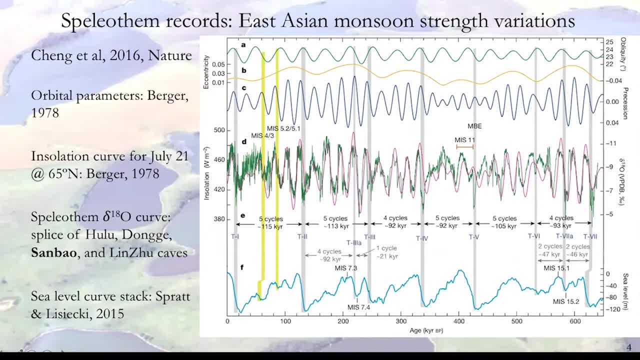 So it's the one dominant factor that affect precipitation amount in these regions. So the green curves you see in label D, that's a splice of multiple caves that are affected by East Asia monsoons and they show good correlation with insulation curves. 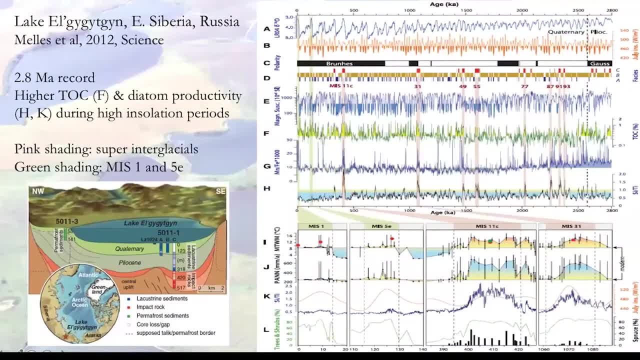 Okay, some of the really long lived lakes. Lake Agigeten- This is a crater lake- has a record going back 2.8 million years And I tried to stretch the record as much as I could horizontally And you can see that the total organic carbon. 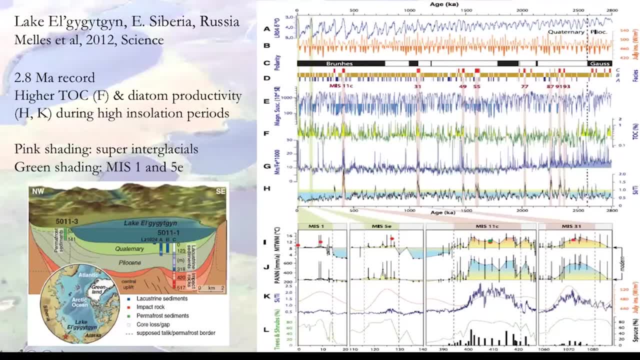 and diatom productivity are high during the high insulation periods And in some periods are showing super interglacials, with mean temperature warm months reaching over 10 degrees in location in Siberia. that's quite amazing. Okay, now back to what factors? 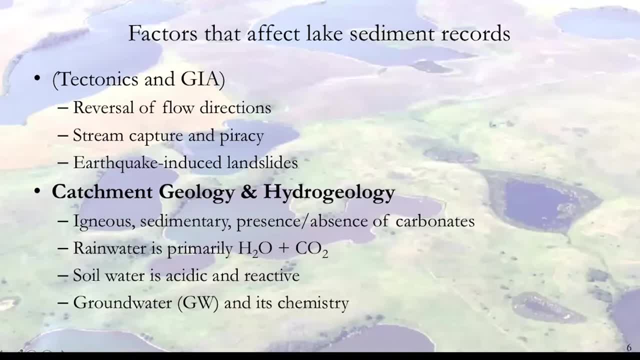 like sediment records. So tectonics and isostatic adjustment, It can reverse the flow of water. If the lake is long, north, south, it can cause stream capture, piracy, earthquake induced landslides- All those things can change to hydrology. 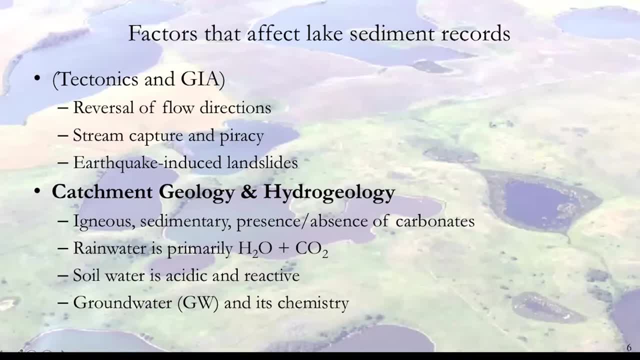 Okay, but the big factor in small lakes is catchment, geology and hydrogeology. So what kind of hydrology, What kind of hydrology? So what kind of bedrocks do you have? Are they carbonates or not? Okay, because rainwater. 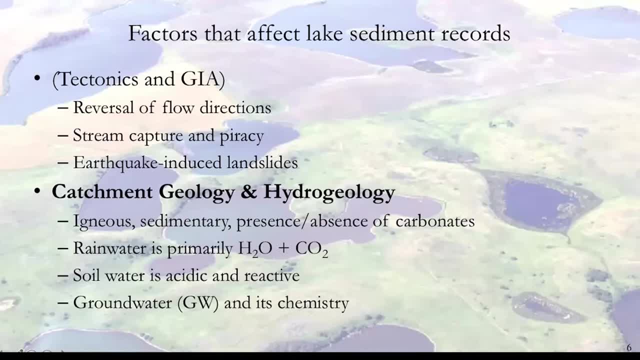 which is the ultimate source of lake water, is primarily just water and carbon dioxide, So it's a very weak acid. Okay, as when rain falls on the ground surface and starts to percolate through soils, soil water, soil is very acidic. 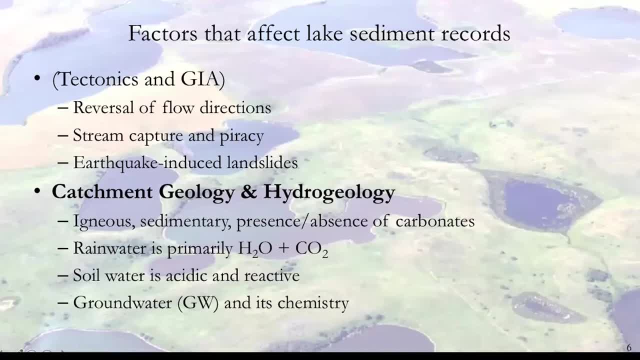 because of all the respiration. So the water becomes even more acidic and more reactive, So it can do quite a bit of weathering And then, once it enters below the water table, be a lot of weathering reactions, or you might call rock water interaction. 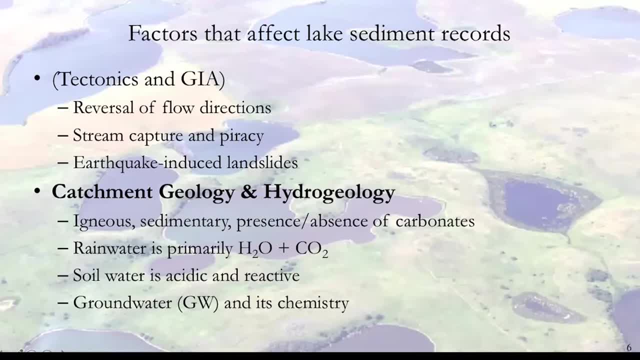 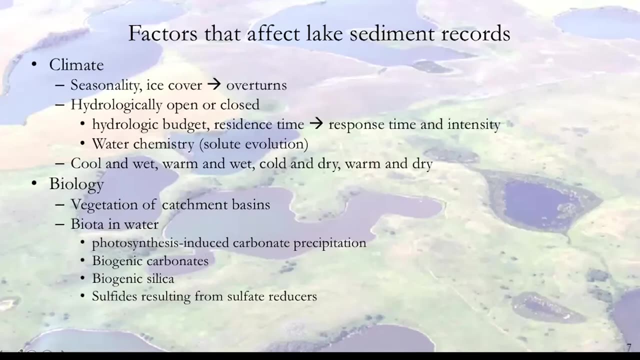 that brings in cations and anions from the rock that the water is flowing through, So it's no longer just the water and carbon dioxide. Okay, climate also affects the lakes. Seasonality: is it mild Temperature all the time, or is it continental, with hot summers and cold winters? 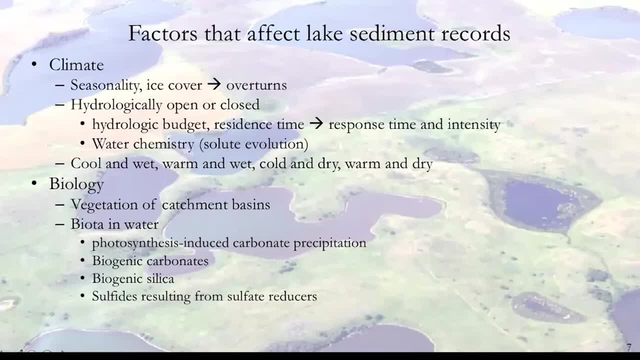 Does it freeze in winter, So it affects the overturn of the water column. Is it hydrologically open or closed? Okay, if in very wet places you don't see many lakes because you just see streams, it's hydrologically open. 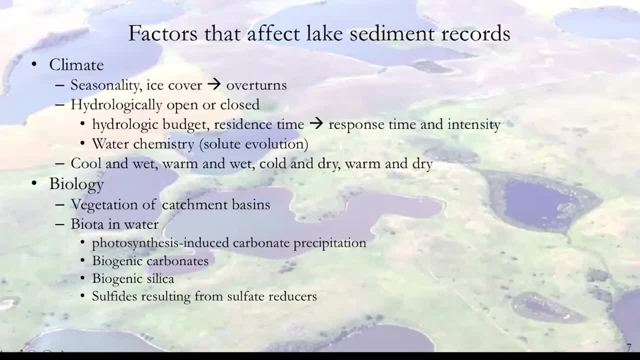 Whereas in semi-arid locations we see a lot of hydrologically closed lakes. Okay, So, whether it's open or closed, that affects hydrological budget, residence time, which in turn affects response time and how intensity changes are recorded, And, of course, water chemistry in hydrologically closed lakes. 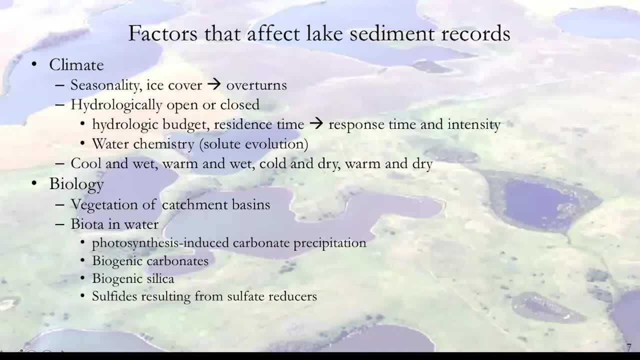 water evaporates, leaving solutes behind, which makes the water more brackish and saline? Okay, And types of climate make a difference And also affects sediment records. What kind of vegetation is growing in the catchment basins? Okay, 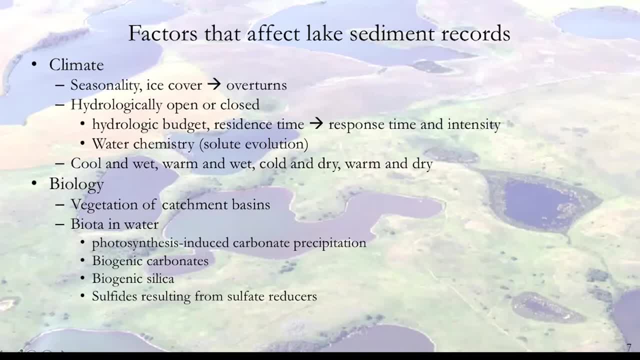 For instance, conifers are well-known for turning soil acidic so that more acidic water comes into the lake basins. Okay, Biotic in water itself, Okay, Algae will induce carbonate precipitation when it's photosynthesis reactive Bionetic carbonates. 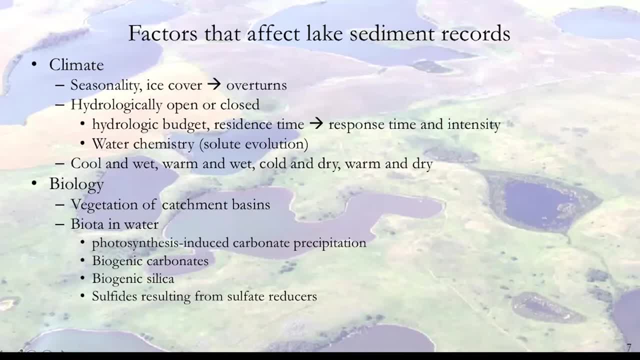 Okay, Ostracods for one Snails. Okay They take, dissolve the calcium and bicarbonate out of water to make calcite, the aragonite, Biogenic silica from algae such as diatoms, And you have soil reducers. 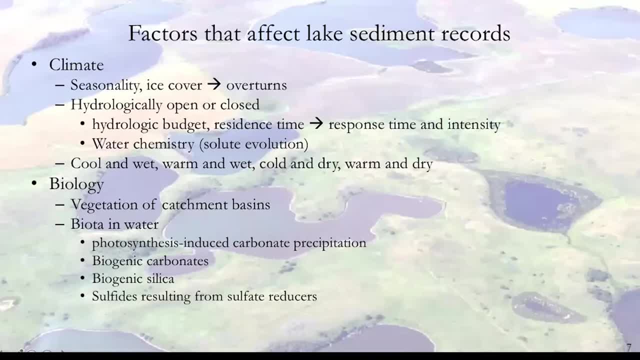 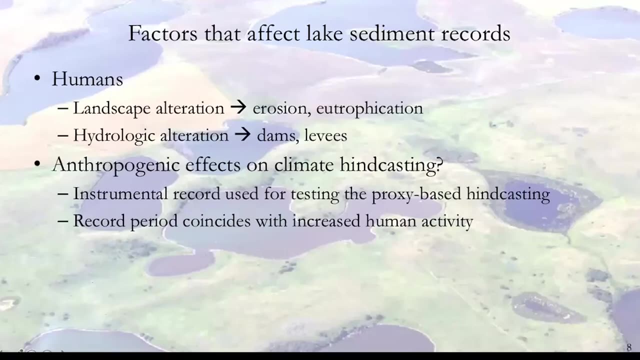 We make sulfides and that's left in a sediment record. Okay, Humans also affect the lake sediment, especially in North America. When Euro-Americans came in, they cut down the trees, So they turned over, uh the prairie and increased the erosion uh. 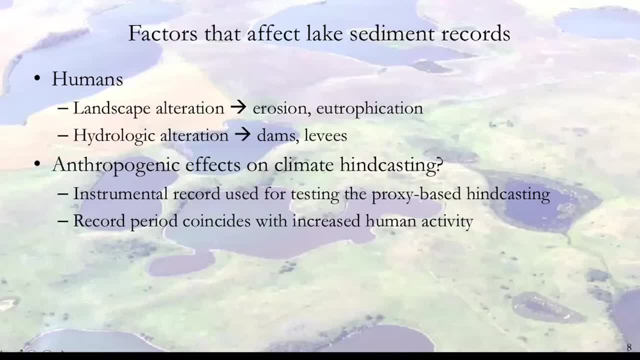 and then you know increased eutrophication of the lakes. Uh, if they build dams or levees, it also changes hydrology. Okay, And the one of the big problems is anthropo, anthropogenic effects on climate hindcasting. 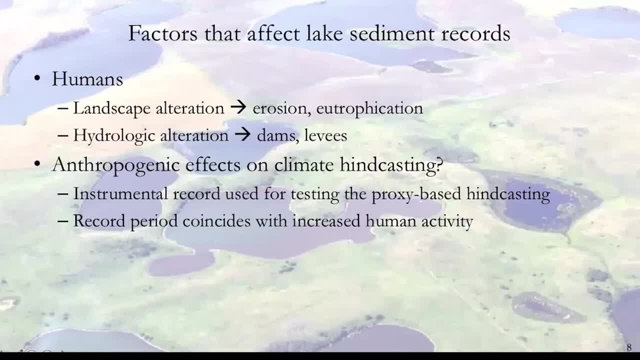 Okay, We often um do try to calibrate using instrumental records. Okay, Instrument records start when human records start. Okay, Instrument records start when human records start. Okay, Instrument records start when human records start. Human effects become really important in North America. 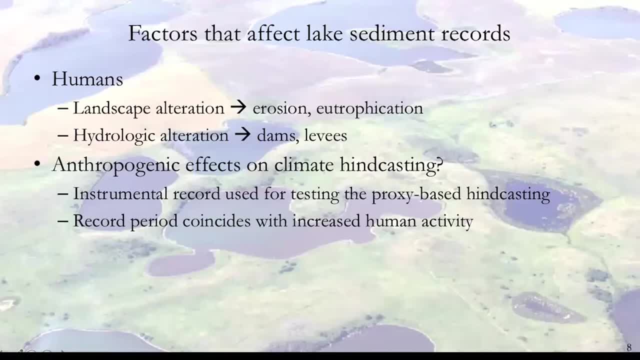 Okay, So what we're using for calibration may not be all that good If you think about what sedimentation may have been like before people came in and, uh um, mucked up the landscape. Okay, So what do we use as proxy records? 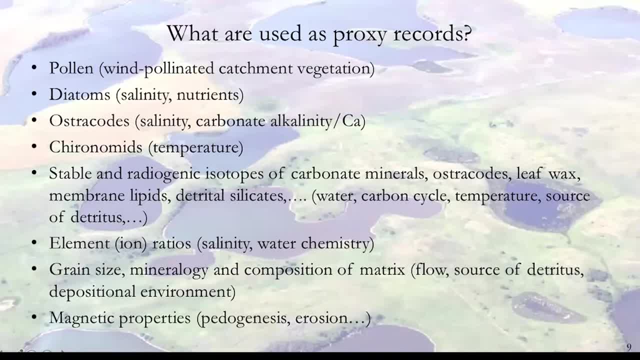 This is not a list, Like Poland, So we use- we use- a proxy record. as we said, it's not a list. we use wind pollinated catchment vegetation Insect. pollinated pollen are usually too heavy, They don't get carried by wind, So it's wind pollinated vegetation Diatoms- okay, so they're. 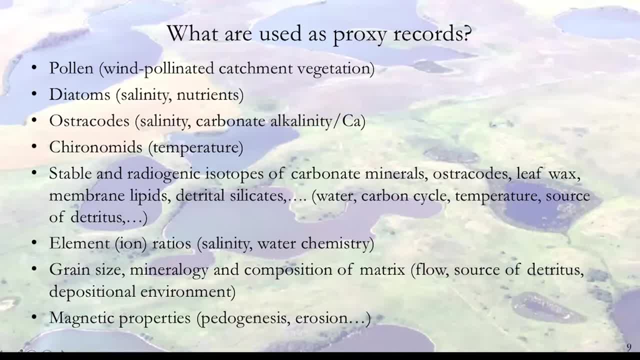 used to reconstruct salinity and nutrient levels. Ostracods- okay so diatoms are plants, Ostracods are animals Often used to reconstruct salinity or carbon dioxide to calcium ratio. So it's one of the few proxies that can actually tell you something to water chemistry, in addition to just. 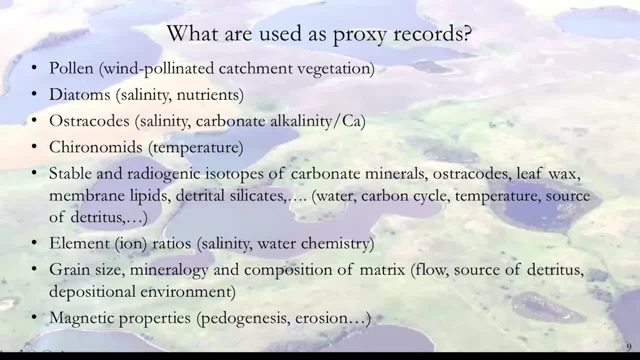 concentration ions. Chironomids have often been used as temperatures. These are non-biting midges- and, of course, a whole bunch of stable radiogenic isotopes or carbonate minerals, Ostracods, a whole bunch of things. You can try to say something with the water or carbon cycle. 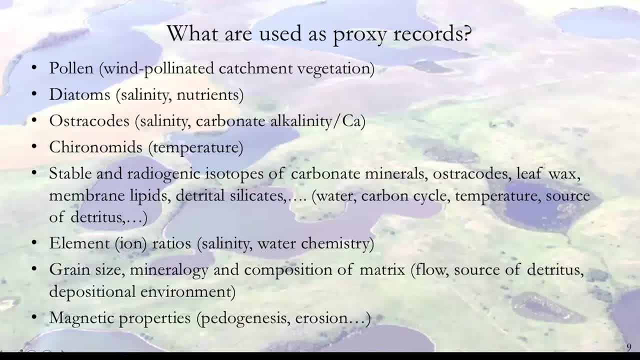 something about temperature, Sources, detritus, et cetera. a whole bunch of applications and possibilities. Element ratios: okay. something about salinity, water chemistry: okay. we need something that record element ratios, okay, And we can. we tend to forget to look at the matrix itself. but the grain size? 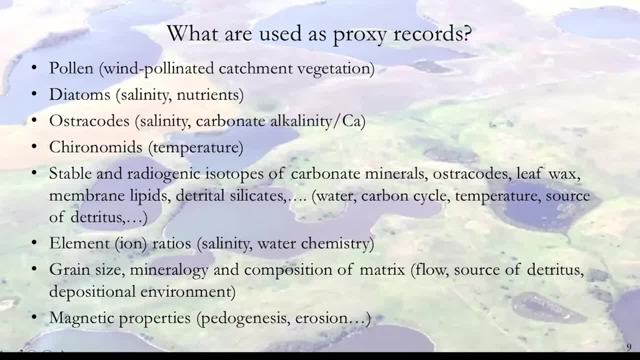 mineralogy, composition of matrix. that tells a lot about strength of the flow. River water has an impact. It's very important A source of detritus, what kind of deposition environment was present, And some people use magnetic properties so they can say something with the petrogenesis or erosion. 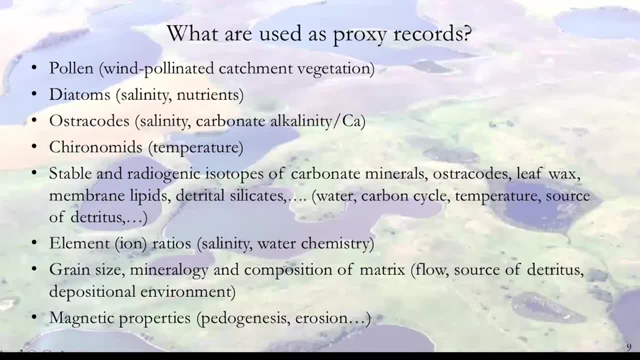 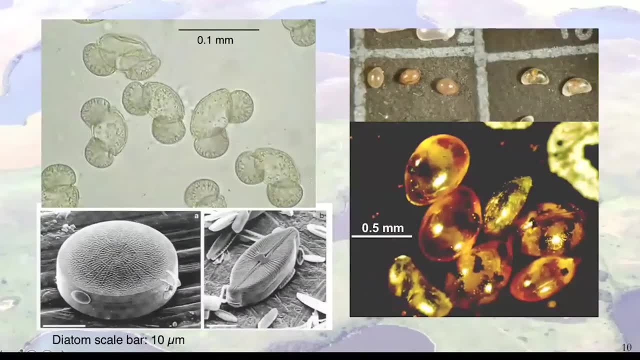 that bring magnetic minerals into the lake water, into the lake sediments. Okay, just a few examples of biological proxies: On the left is pine pollen. So the scale lower left to our central pond is pine pollen. In the lower left two are central pollen. 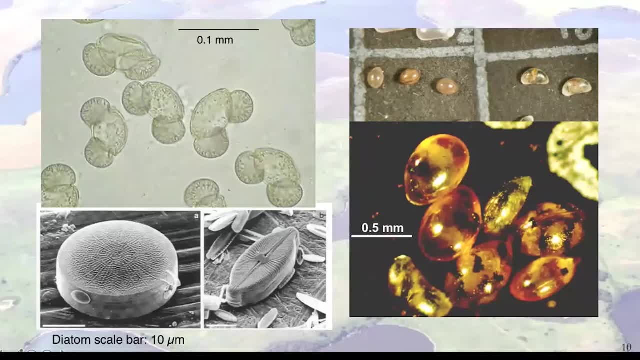 In the upper left are central pollen, In the lower left two are central pollen, In the lower left is central pollen and penate diatoms. diatoms scale across 10 microns. And on the right hand side our ostracodes of diagrams are dead ones. 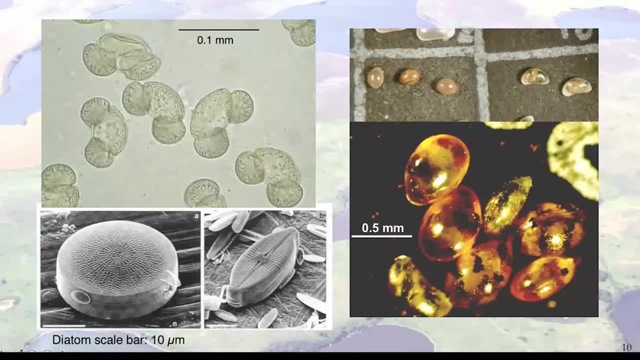 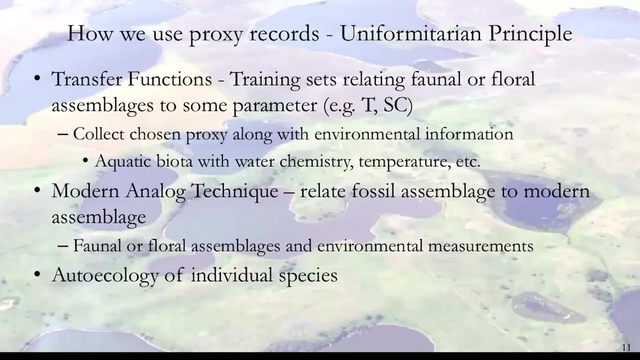 And then lower right is live ostracodes, which actually have patterns and whatnot. All the pigments get destroyed after they die. Okay, so how do we use proxy records? A uniformitarian principle is used. A transfer function is a very popular method. 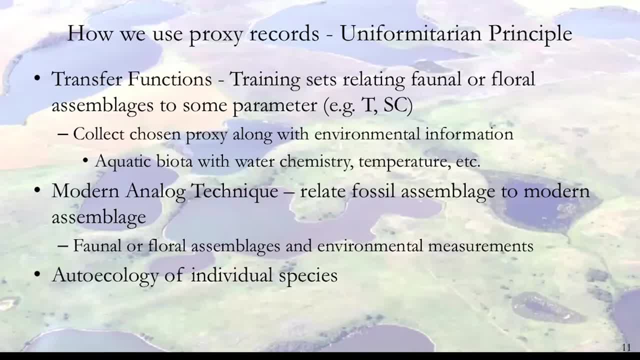 We make mean sets that relate to formal floral and stem pattern. Okay, so you might collect a whole bunch of diatoms from many lakes in general region, All the environmental information, or you might collect water temperature et cetera. Okay, or modern animal technique. 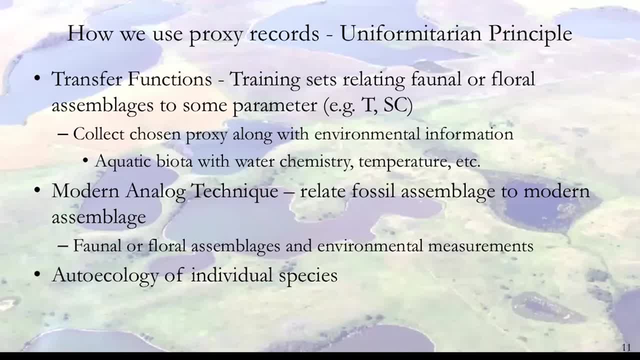 we relate fossil assemblage to modern assemblage, typically used with vegetation, but with other things as well. Okay, and in both of these techniques, there's an assumption being made that we already have an idea. what is the important environmental factor? 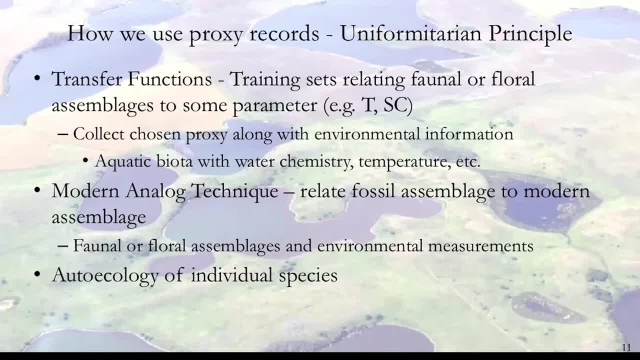 that is affecting distribution or presence, absence of different species, say of ostracodes or diatoms. If you don't know what they are and are not measuring it, then no matter what kind of ordination you collect, you're not going to find what is affecting. 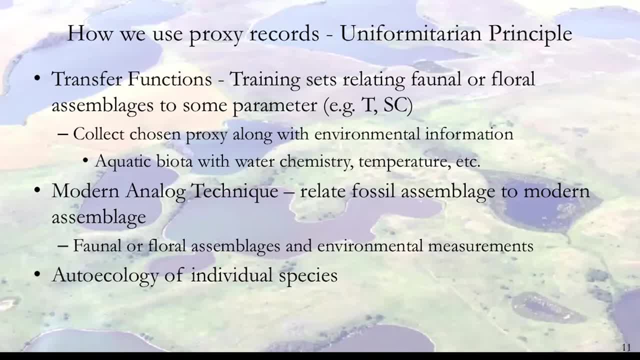 the distribution of the fauna or flora that you're studying, Okay. the third one that I rely on quite a bit is is all ecology of individual species. Okay, so it's complete life cycle, when they molt, when they hatch, where they bloom. 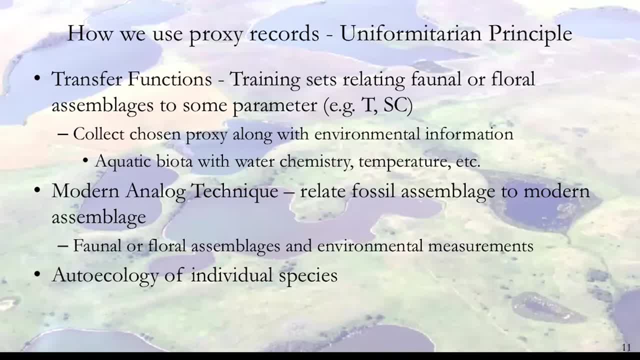 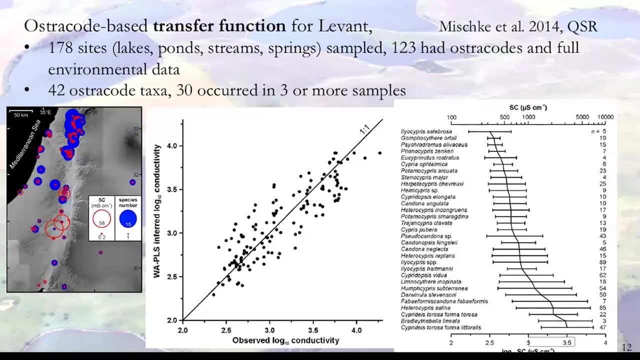 and how they react to different environmental factors. Okay, so here's an example transfer function by Stefan Mischke and co-authors. So it's Levant: 178 sites were sampled and 123 had full environmental data And ostracodes. they were kept. 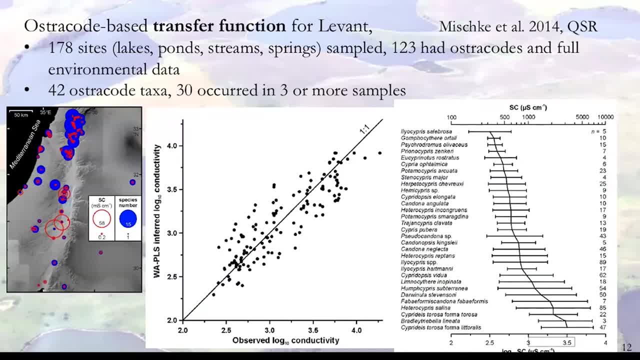 And then from that, from 42 ostracodes, and of that, only 30 occurred in three or more samples. Okay, so we don't want to end up using something that only exists in one location, which may have been brought in by the aquatic bird. 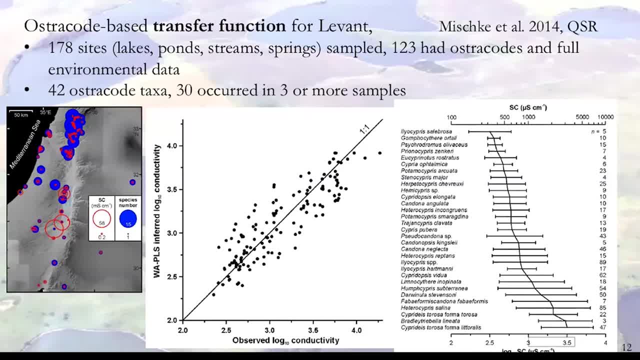 and it's not really native to that lake, So those are eliminated. Okay, so on the right-hand side you can see 30 species with their range of specific conductivity, And so, after the ordination, specific conductivity was found to be the dominant factor. 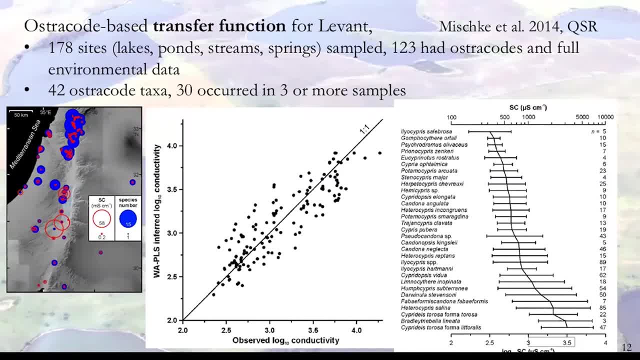 in distribution of these species. Okay, and then a weighted average, partially squared method was used, And then a middle figure shows how well the training set works against the actual measured specific conductivity. Okay, now this one was used to reconstruct the temporal changes. 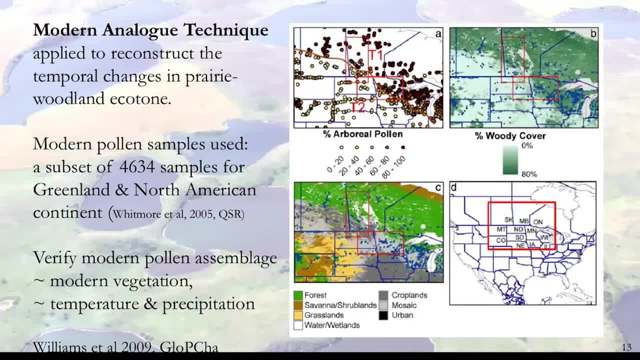 in prairie woodland ecotone. So on the figure A- it's the brown line- is the difference between areas to the northeast, which has many more trees, and then to the southwest, which is, you know, which is more prairie. 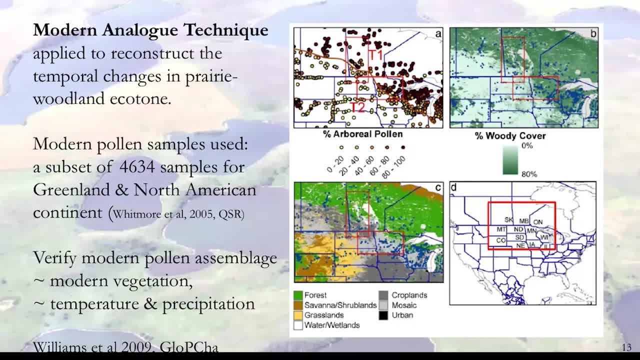 Figure B is from the remote sensing data. Figure C is what the modern vegetation looks like. But you verify that modern pollen assemblage looks like the actual modern vegetation and that there's a good correlation with temperature and precipitation. Okay then, with that you can take sediment core. 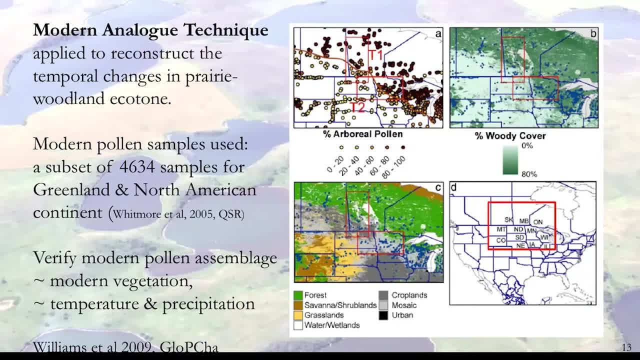 from some area within this region and then start looking at the pollen assemblage and compare against modern analog. Okay, so you might find that 6,000 years ago the pollen assemblage is similar to what exists in some area to the south of the current location. 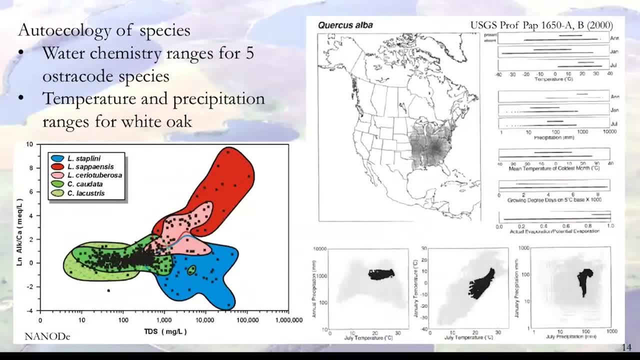 Okay, So here the pollen is not going towards the east coast. These are the new ones you'll see on the left, so that's why you'd need to take all of that into account, So that's why it seems nice to walk the path. 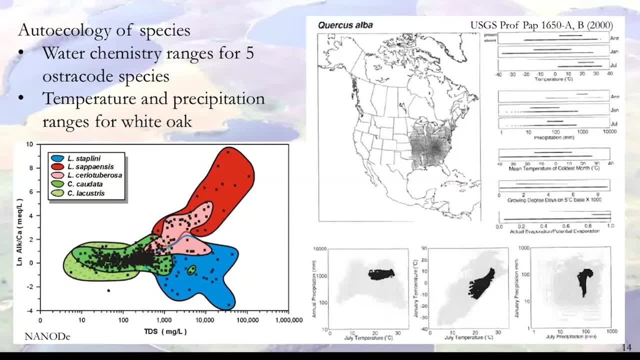 where they've already found this And look, you also have some of that sediment and it's very likely that it's not going to be the same place. However, if you look at the bottom, you might see some of that sediment. 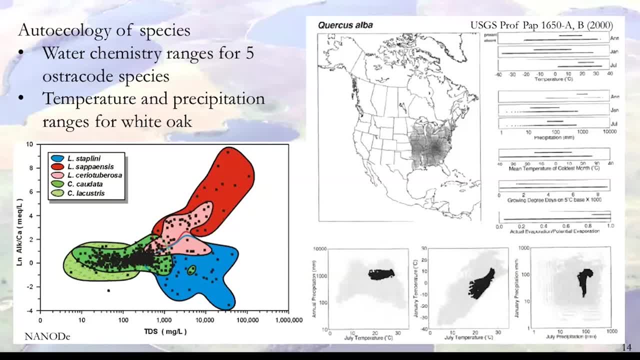 waters that have low alkalinity to calcium ratio and some are high alkalinity to calcium ratio, and in dilute water they're all staying sort of near alkalinity to calcium ratio of one. Okay, and then USGS has a fantastic record looking at temperature precipitation. 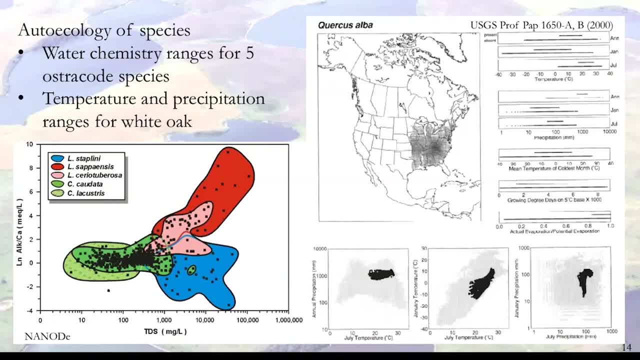 range for a whole bunch of trees, both deciduous, and then for white oak. So the faint gray areas are all the climate combinations that are found in the northern area. Okay, and then black parts are indicate where white oak is found today. Okay, going back to the finality problem, which is not just for small lakes, but I think it's. 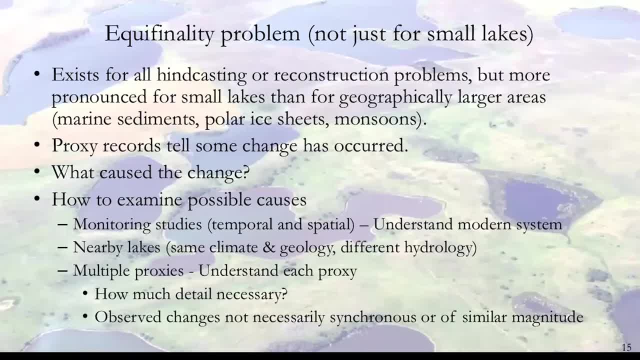 particularly dire for small lakes. So existing no heimcasting construction because nobody was there when changes were taking place, looking at finished experiments and trying to figure out how to do it. Okay, what happened? Okay, and small lakes were much. they're much more influenced by what's going on in the catchment. 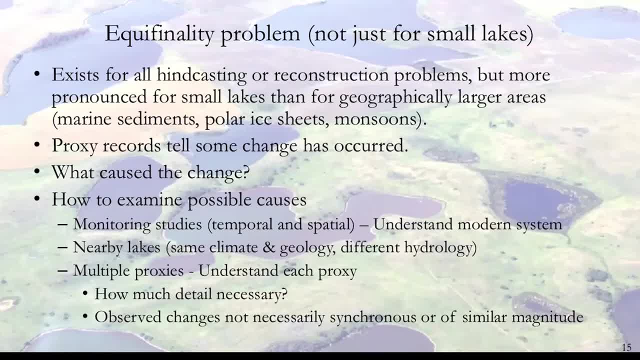 So compared to marine sediments or polar ice sheets and monsoons, equi finality is a much more serious problem. Okay, so we can tell some changes occurred, but what caused the change? that's a whole nother problem challenge. So how do you examine possible causes? 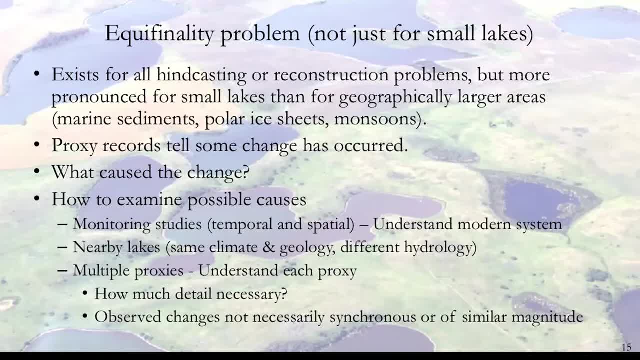 Okay, one of my favorite- if you can relate to extent up with monitoring studies, Temporal, is what I've done with training sets and analog studies. they're looking at spatial variants, so they're sort of substituting space for time. So try to understand the modern system as 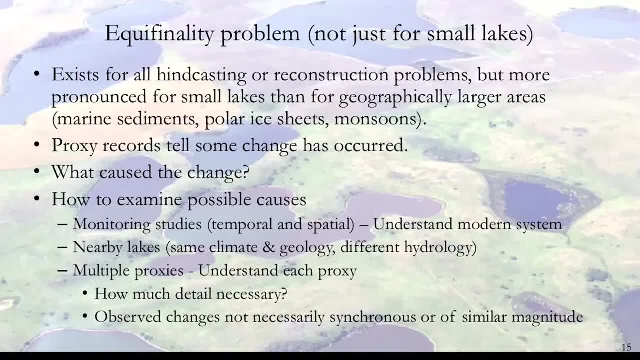 much as possible. So you might look for lakes in nearby lakes, you might look for Arab lakes from saying clam and geology, but with different hydrology, to see how they might react differently, and then use multiple proxies. Understand each proxy to detail. do you have to understand for each proxy, and and what we can. 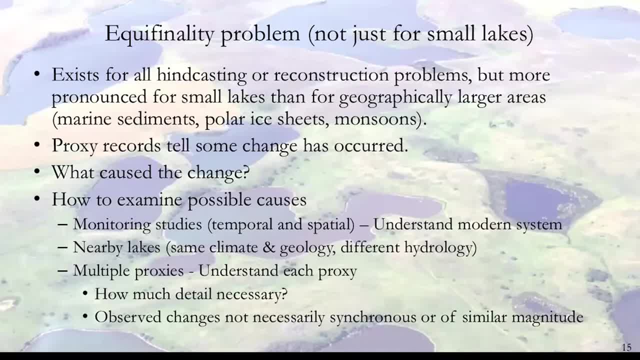 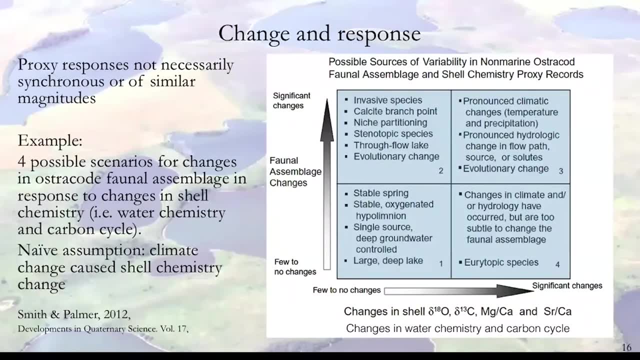 deserve change, necessarily synchronous or of similar magnitude. So I'm going to move around a little bit here. So, for example, here's Osterquartz. so it shows four possible spheres for changes in Osterquartz form of assemblage in response to changes in shell chemistry. 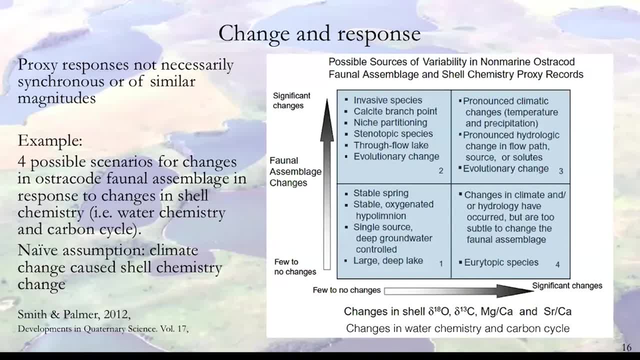 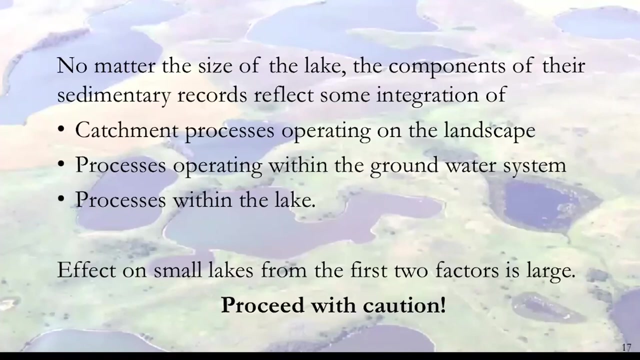 Here the assumption is that shell chemistry is related to water chemistry and there's a delta C13, a current cycle. So an assumption being made here is that climate change causes shell chemistry to change, which may or may not be true. So take-home message- I'd like to take you away- is no matter the size of the lake there's. 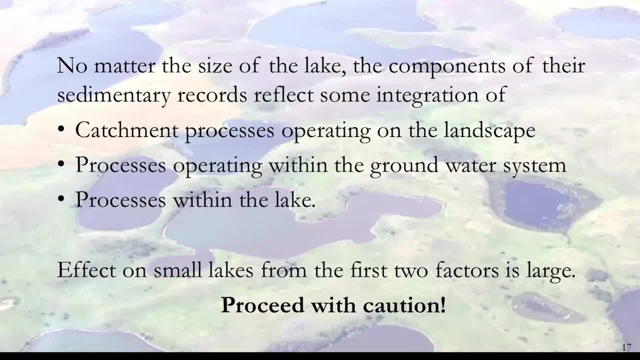 three things that are going on: catchment processes on landscape within the groundwater system, which I think it's my favorite Confounding factor. groundwater, and then processes in the lake. So effect on small lakes from the very large. so proceed with caution when you're trying. 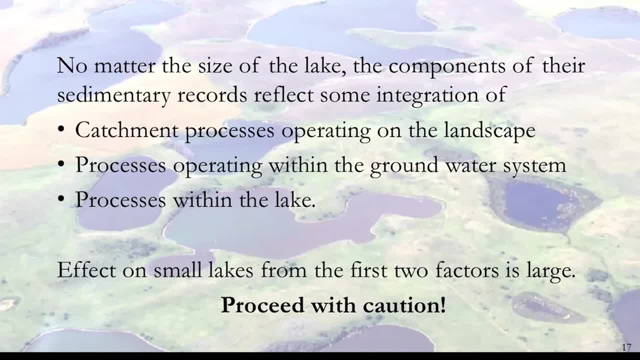 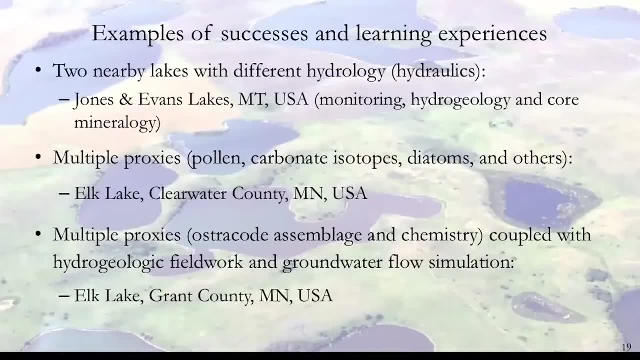 to reconstruct or model past climate or environment using sediment from small lakes. Okay, so I'm going to use three examples so I can have time to finish them. So first I showed nearby lakes. Different hydrology, actually permeability in the aquifers. 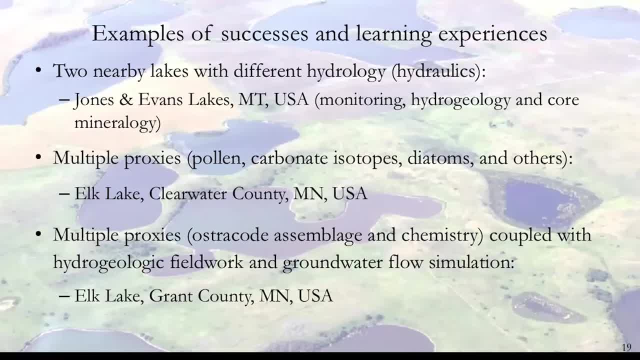 So lakes from Montana. Second one's an example: multiple proxies, the Elk Lake and Clearwater County. And the final one is a different type of multiple proxies which is coupled hydrologic fieldwork and groundwater flow simulation, Also from Elk Lake, but it's from Grant County, Minnesota. 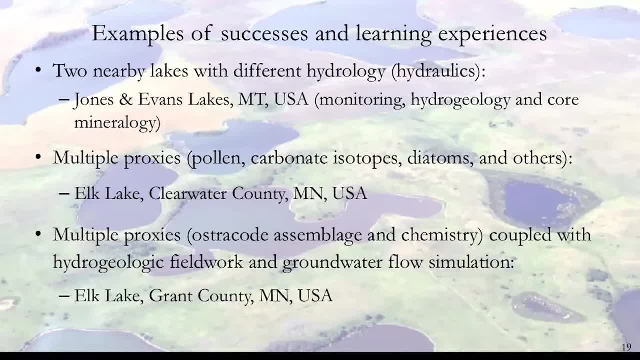 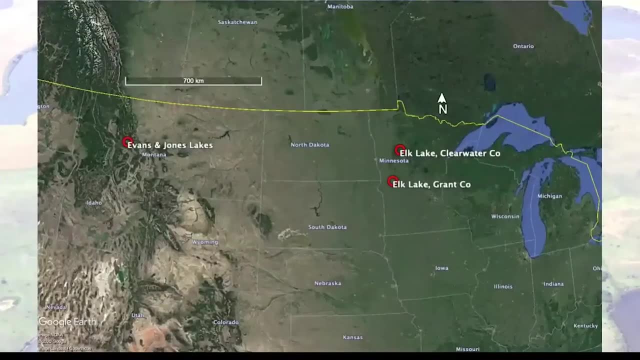 Every county in Minnesota has at least one or two Elk Lakes in addition to Cedar Lake, Long Lake, et cetera. So I need to specify which county they're in. Okay, so these are the three lakes: P minus ET precipitation, minus evapotranspiration. 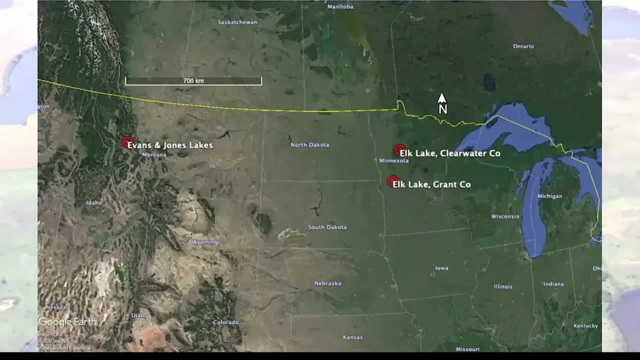 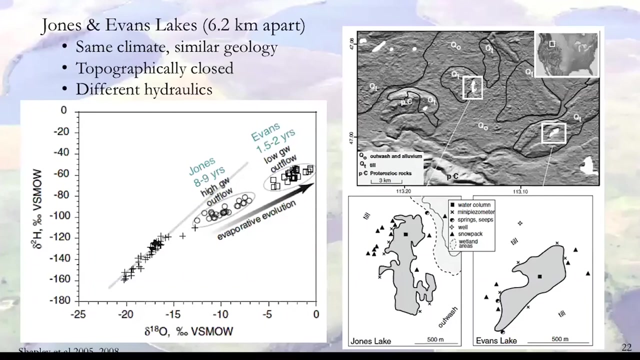 is usually positive. Elk Lake- Grant County's P minus ET about zero. Evanston Jones Lake's P minus ET is negative. Okay, So the lakes are six months apart, have the same climate, geology's similar, although Jones is located with a lot of evapotranspiration, outwash and rubium, whereas Evanston's later. 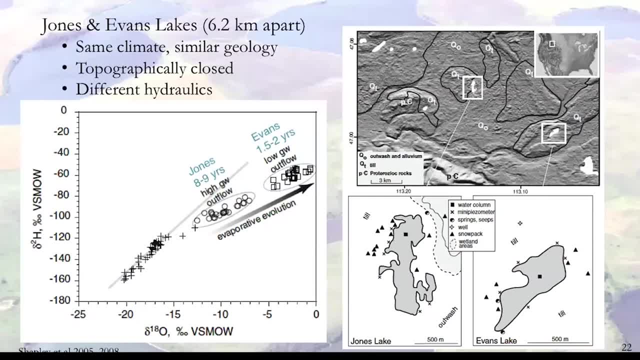 hole in Glacier 2, which is much lighter, with much lower permeability, And you can see- I've reversed- that Jones is .5 years and this is .9 years. Okay, So the Okay. This is showing much farther evolution from the precipitation fall in the area. 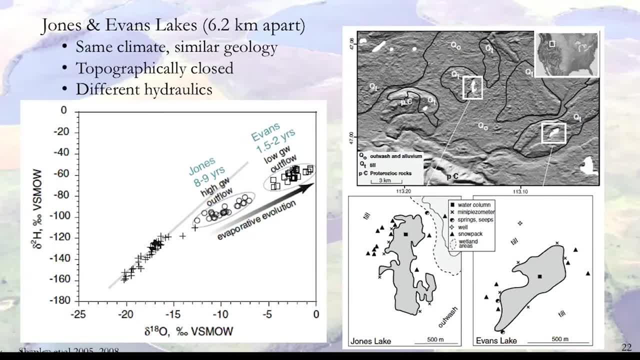 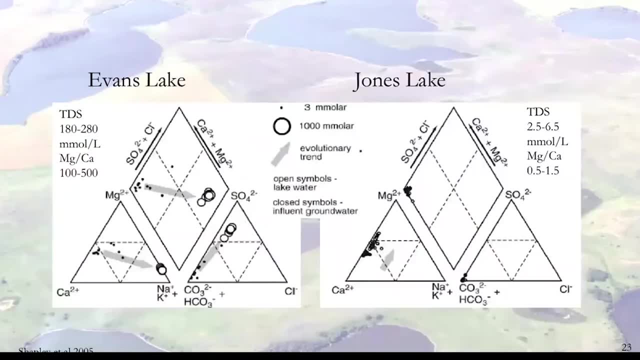 Okay, This is montrer just. Zeous lake has solid to Kn barbecueик, which is quite high, because all the calcium that comes in through groundwater is immediately precipitated out as a raganite, so that lake water has no calcium left. 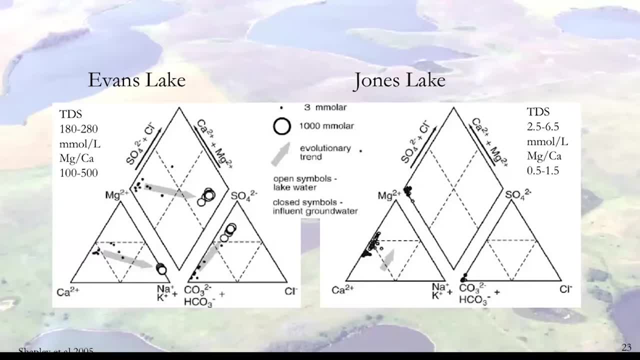 SGT минут快 starter corresponds To half of the water sources existing underground in the lake liter scale, thanks to an set of other balls of oxygen. The maximum of it there is yanit Dave from the Ref MUSICE Fson después de Viz, shoulders 1282.. 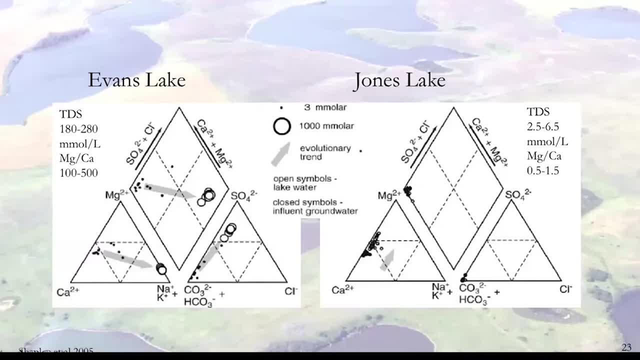 So this layer has to be Obviously me. The larger portion is beta-tповiel mountain, So that's it. So this is the ascending principle: enrichment. but when you look at carbon dioxide quantity over calcium ratio, it's still increasing. 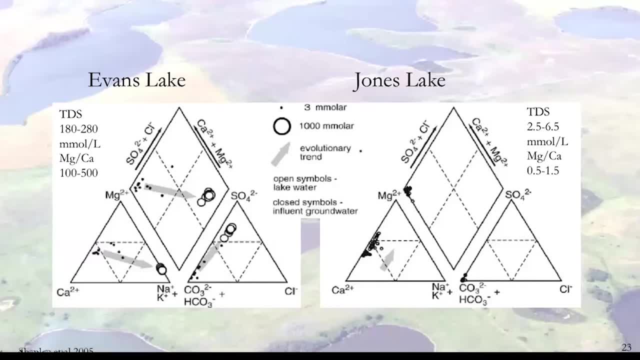 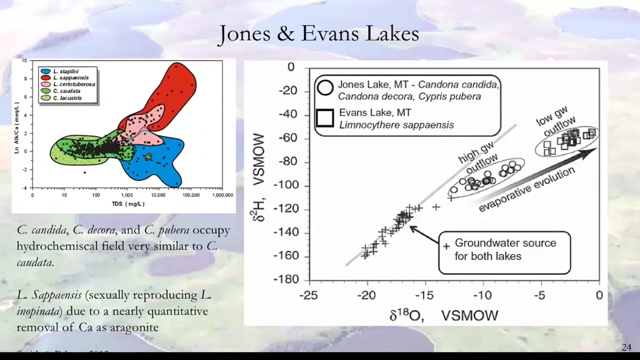 because calcium removal is so complete In Jones Lake, with a shorter resistance and much higher loss of leg wall and ground resistance, TDS remains quite dilute and its concentration also remains quite low. Okay, and what you see is that the Jones Lake, because of its water chemistry, has types. 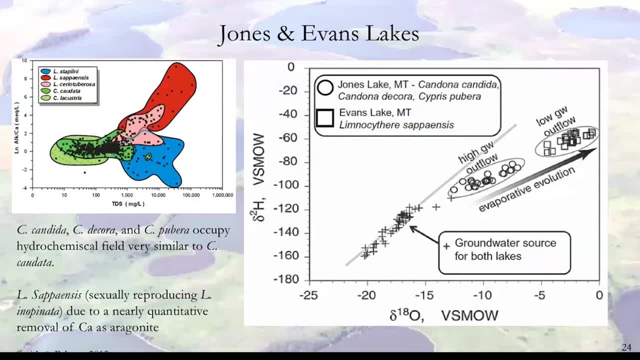 of masticators that are in the saline zone, dilute waters, whereas Evans Lake has some of these water types that are in the saline zone. So if you look at the testicles' physics that can do a lot. So you get the feeling that these two lakes may be different climatic regime. 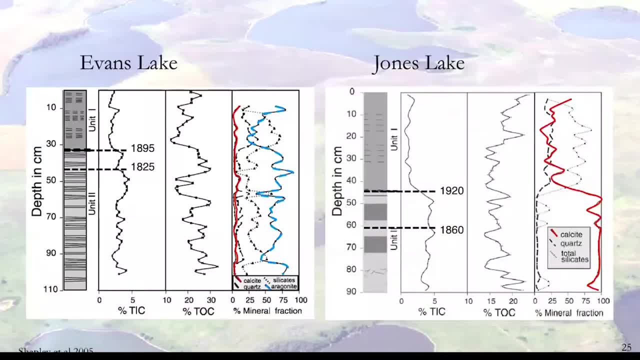 And both lakes show consistent pattern. It shows the effect of human settlement, increase in erosion. okay, so that relative proportion of carbonate or oestrogenic minerals decreases. okay, so the sense of timing effect of human settlement are recorded in both. but Evans Lake makes you think it's in the arid environment and Jones Lake 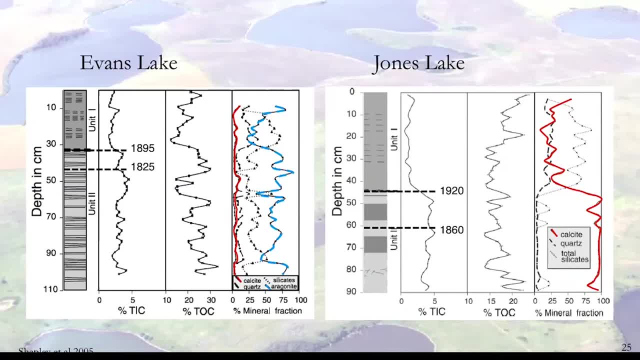 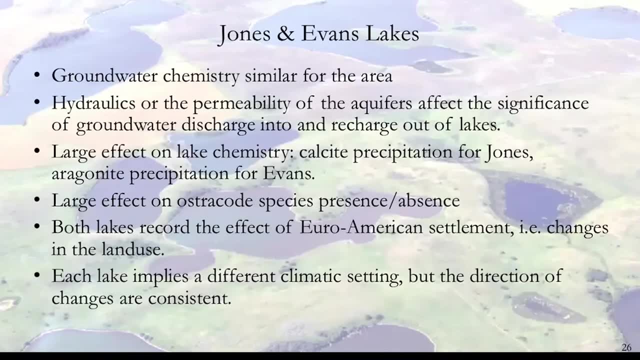 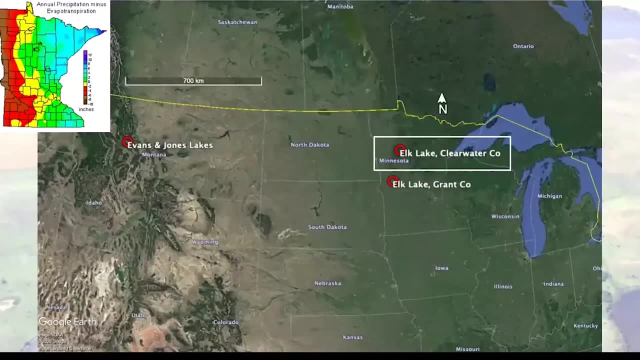 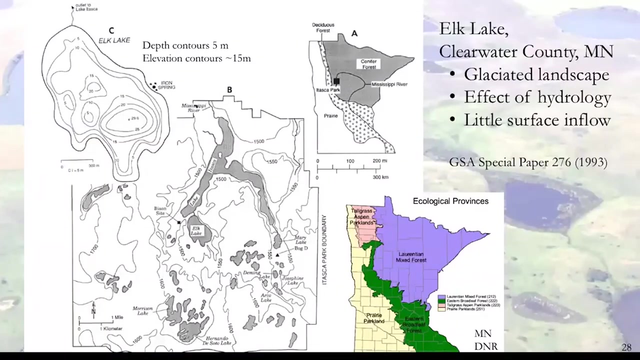 make you think it's in the humid environment. okay, so hydraulics of the aquifers really affect how lakes behave and what kind of sediment is formed. okay, let's move on to our lake, Clearwater County, and so right about here. so it's in the P-ETE positive, okay, and it was studied by a whole bunch of people. 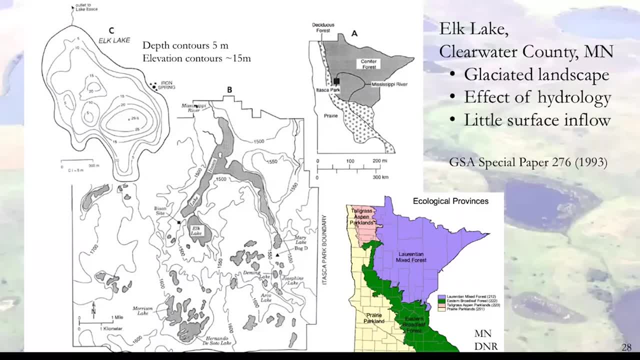 from USGS and from University of Minnesota. all came out in a special paper, JSA special paper 276 1993. it's all black and white, okay, let's move on to our lake, Clearwater County, and so it's in the P-ETE positive. okay, and it was studied by a whole bunch of people from USGS and from University of Minnesota. all came out in a special paper. 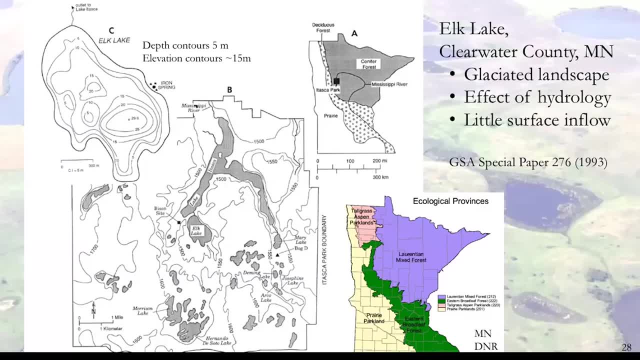 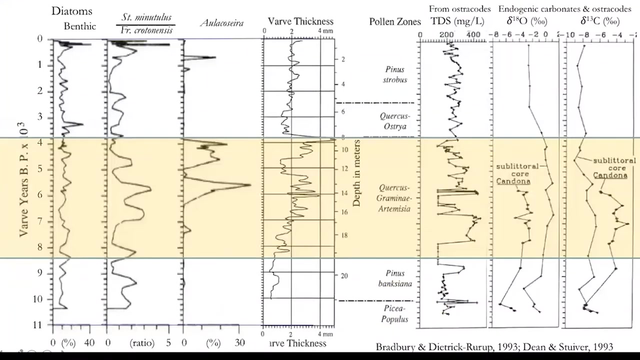 Oh, sorry, i just lost the screen. I can't see what I'm doing. okay, so it's in the P-ETE positive, okay, and it was studied by a whole bunch of people from USGS and from University of Minnesota. all came out in a special paper. 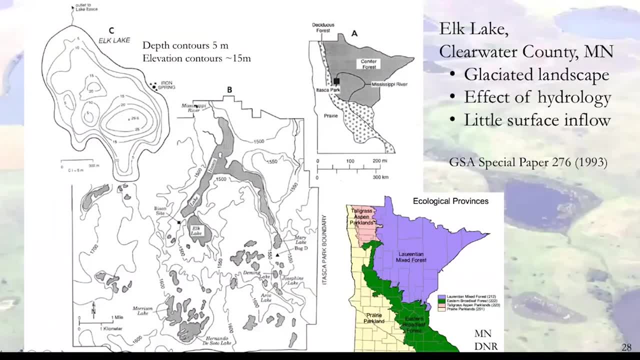 Elk is the source of the Mississippi River, so it's located towards the edge of the Lowlands and the Midwest Forests and the Converse Forests and it's a deep lake and it's permanently stratified at the bottom of the Saguaro River sediment. 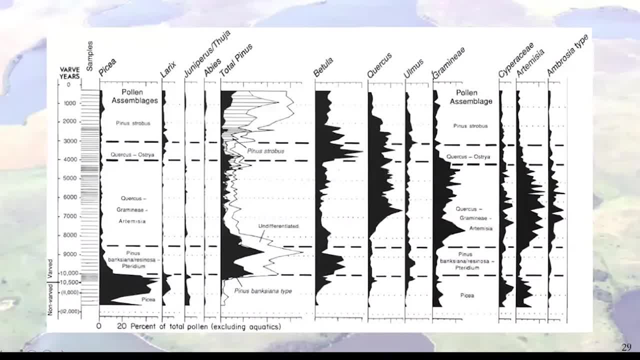 So the chronology is counting. the vast annual conflicts between precipitation And the vegetation is typical of what we see in northern Great Plains: Staghorn trees are taken over by warm drink climate, oak and grass. Sears are washed And then we have birch. 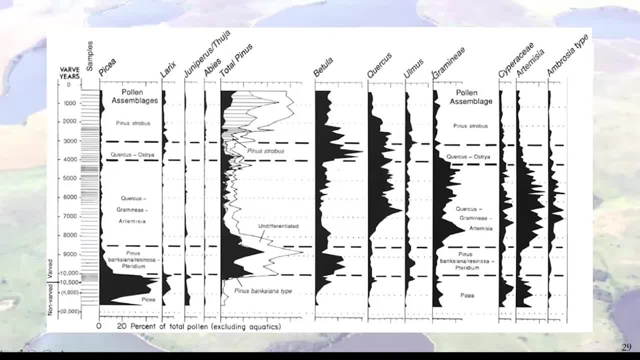 Birch, And then Then here from the forest, we're looking at the jack pine. Okay, so vegetation reconstruction tells you that it came from the early Cold climate, with changing to jack pine and then prairies warmer and drier and coming back to cooler and wetter. 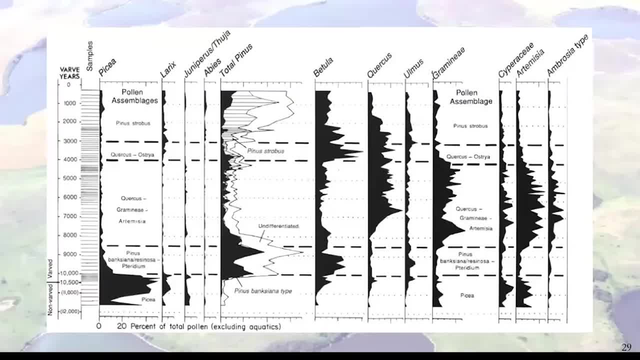 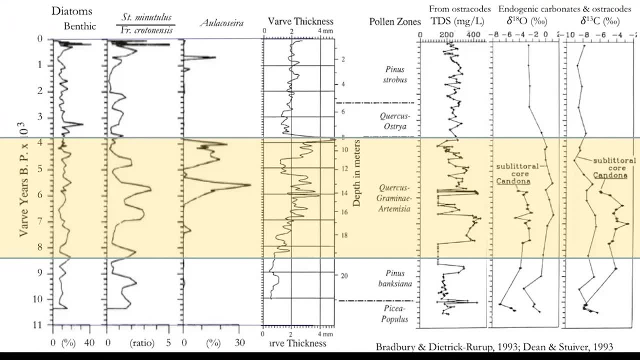 Cooler and wetter climate. Okay, if we look at things that were living in water. first of all, look at diatoms, benthic diatoms- Okay, diatoms are for synthetic algae, so benthic diatoms: you're not going to find them unless enough sunlight reaches. 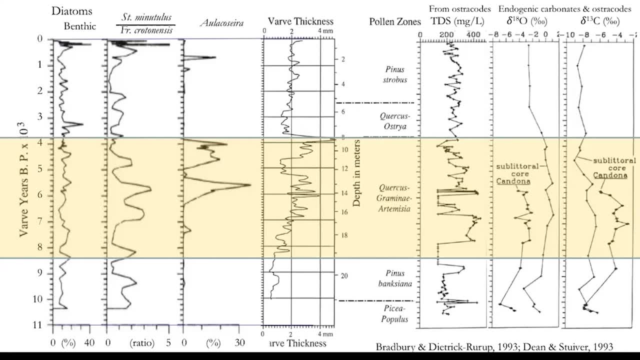 Okay, so the benthic diatoms stay relatively low in concentration, less than 20%. Okay, so the environment didn't change all that much. Okay, and the ratio of Stephanodiscus minutus and Fragilaria crotonensis. that tells you the difference between: 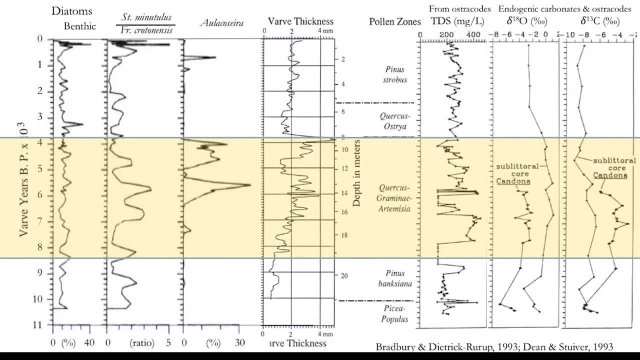 which is preferred by Stephanodiscus, which requires a lot of phosphorous. So when water column overturns, bringing nutrient from the bottom, Stephanodiscus goes crazy, Okay, whereas Fragilaria crotonensis and Prefer waters with, and then lower, phosphorous. 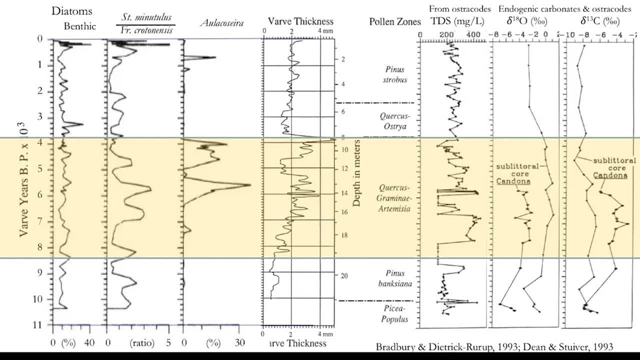 So that bring a lot of eolian sediment that favors Polluxera and Fragilaria. Okay, so during the prairie period there are fewer trees, so there's less shielding from the wind effects, So there's much more mixing. 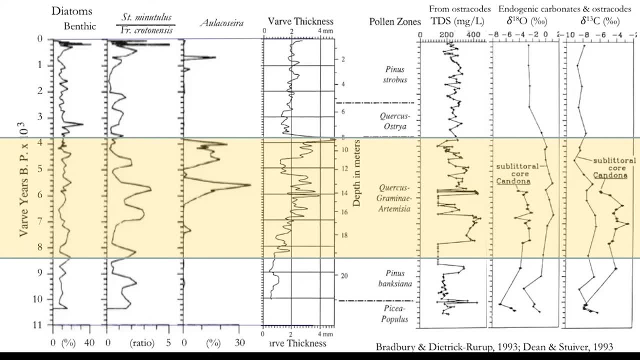 Okay, and from for assemblage modeling says that during the prairie period the dissolved solids are a little bit higher. Okay, but if you look at DeltaO18 of endogenic carbonates in osticards, there's just a little bit of change toward higher values, but not much. 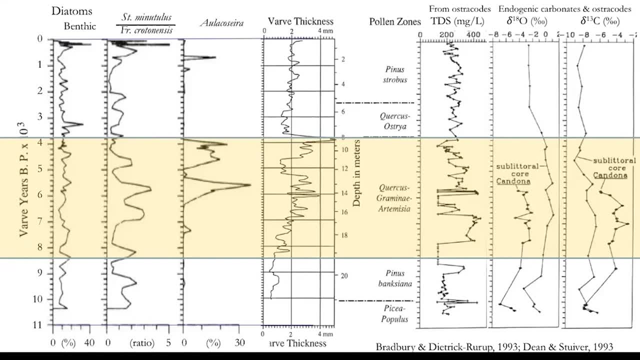 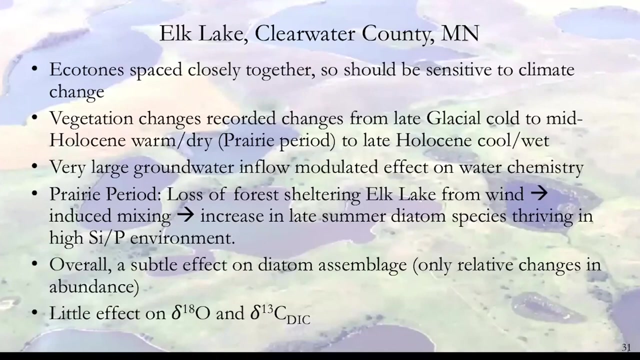 Okay so it's pretty unremarkable. We look at for indicator of water And even though there are relative changes in abundance of different species, they mold wholesale into a different type of environment. Okay so Elk Lake is an area. that's where the eolian comes from. 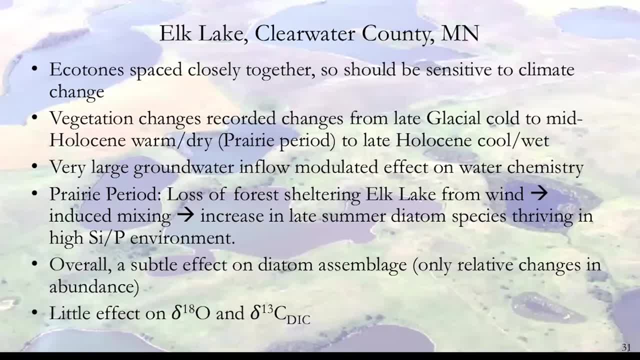 From the mixed forest to deciduous forest. the prairies place really closely together, So you should be sensitive to climate change. And yes, vegetation changed before that, But because of the water inflow, water chemistry doesn't change that much. 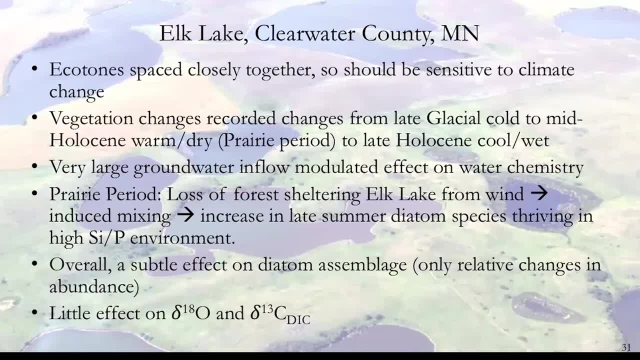 Okay. so what you see is the effect of the loss of forests that shelter Elk Lake from the wind, But overall there's very subtle effect And not a huge effect. Not too nice to observe. Carbon, dissolved carbon- Okay. so last example, 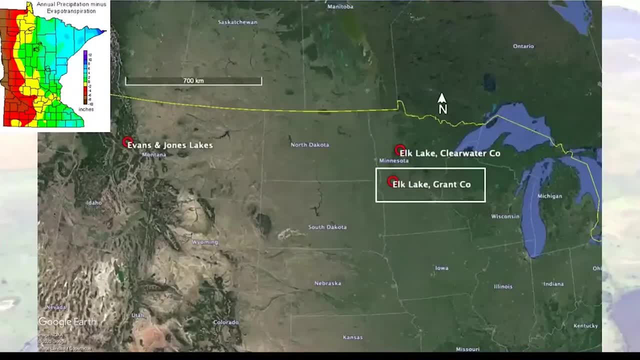 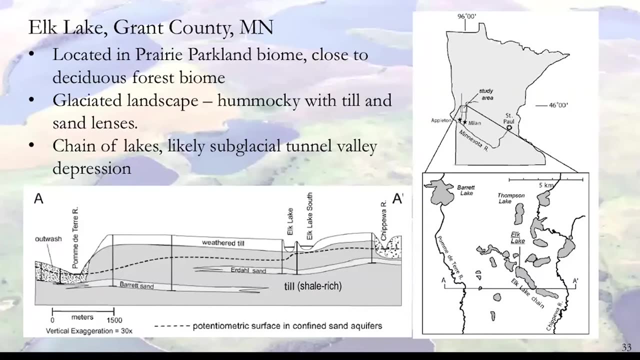 Sorry it's taking too long. Elk Lake, Grand Mountains. This is an area that is close to prairie parkland biome And not too far from the geospores biome. It's a good shade. It's a good shade Landscape. 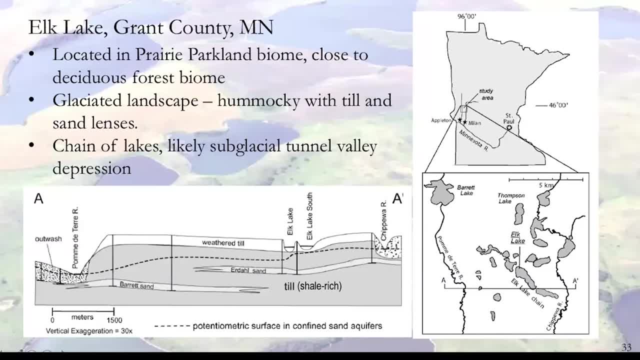 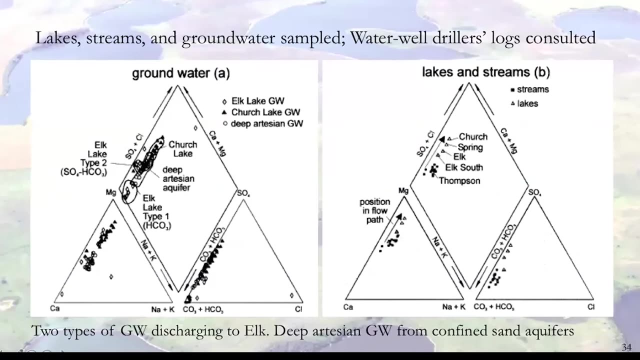 Roots, a lot of chill With some fine sand, And the lakes here have been spoiled. for a sample, We have groundwater from two navigation streams: Elk Lake, Right here. There are two types of groundwater that's discharging. One is dominated by carbonate. 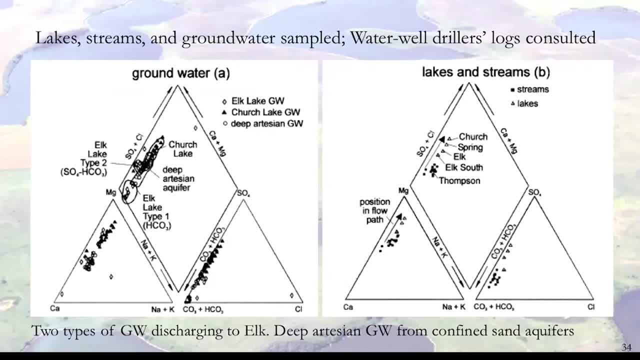 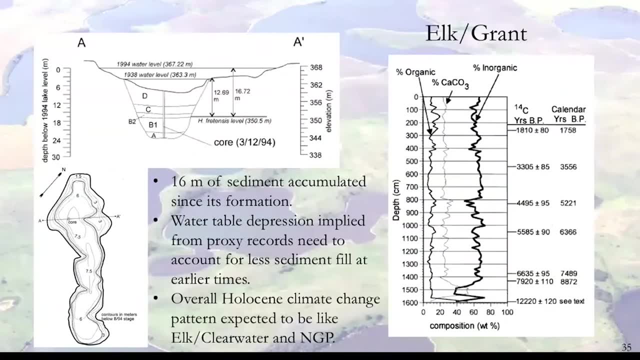 The other is soil. It's dominated by sulfate and bicarbate. Okay, so 60 meters of cement And overall climate change is expected to be very similar to Elk, Clearwater and Northern Great Plains in general. It also causes species abundance. 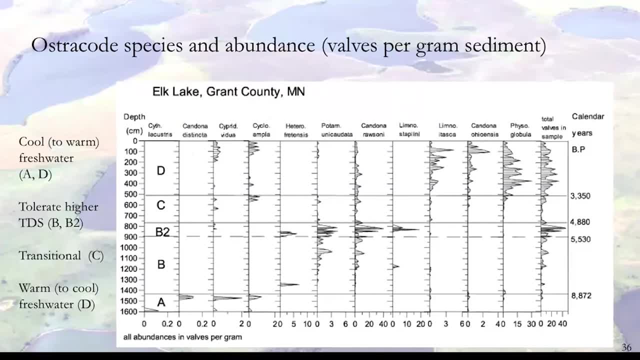 So cool to warm, Maybe warm freshwater species are found in zones A and D. Species found in zones B, C and D And in zone D: warm, fresh, cool fresh water species. Okay, We have isotopes, Calcium. 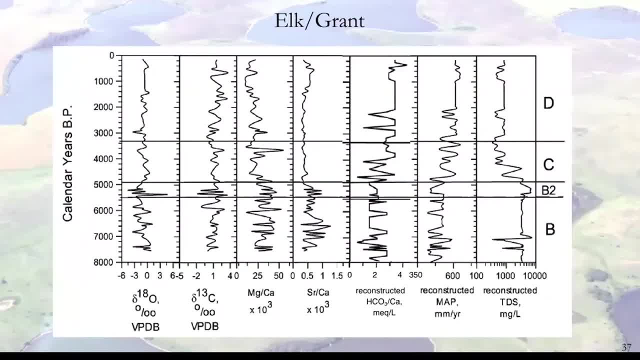 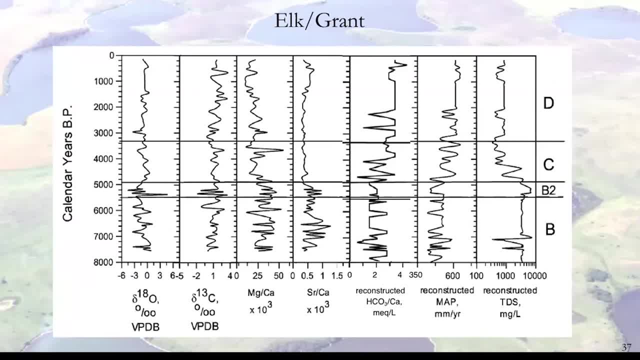 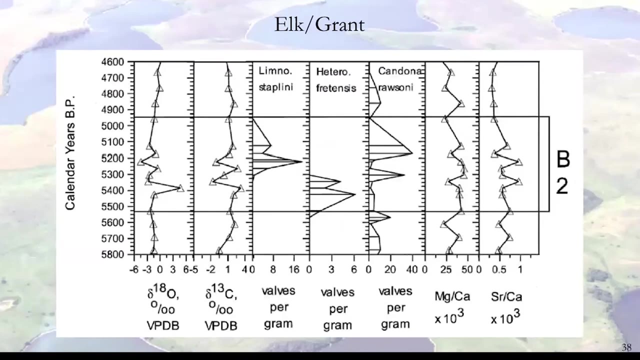 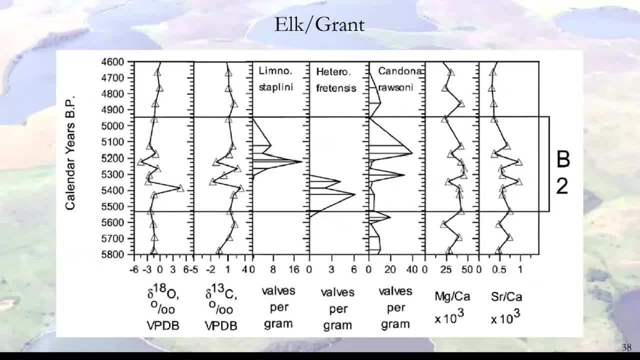 Calcium. Yes, this is the peak of the prairie dry period. We expected the delta weighting to be consistent and high, but we learned low values. Two species, Pneumocystida plunii and heterozygous protensis. 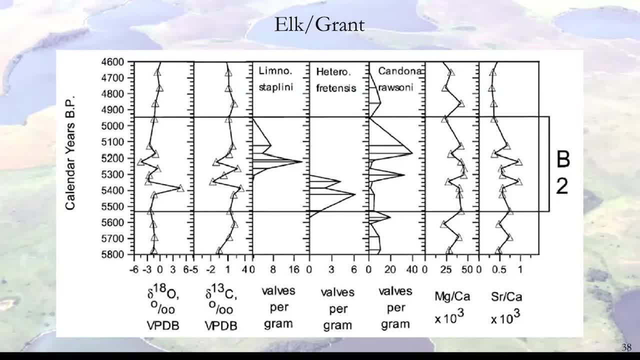 come to rescue when we need to figure out what's going on. Heterozygous protensis like Pneumocystida plunii was in seepage areas, so it indicates that the core location, which is from the deep hardware lake, had so little water that the groundwater table was at that level.